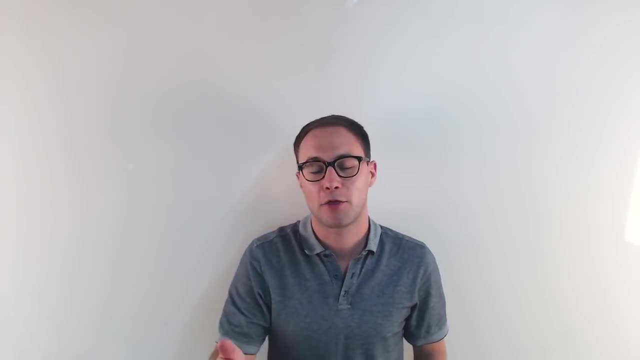 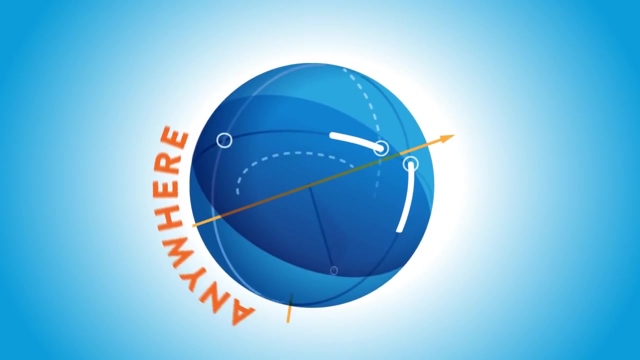 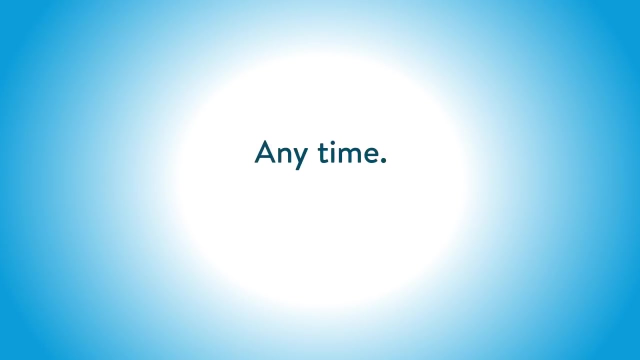 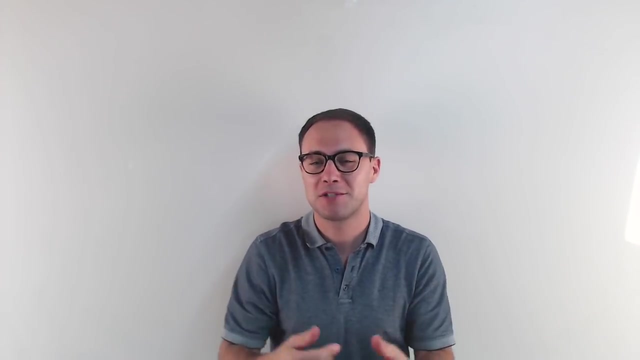 A wall in your room is 5.6 meters by 3.2 meters, A small can of paint will cover about 20 square meters. Do you have enough paint to paint your wall? Welcome to Anywhere. Math, I'm Jeff Jacobson, and today we're going to talk about multiplying decimals. 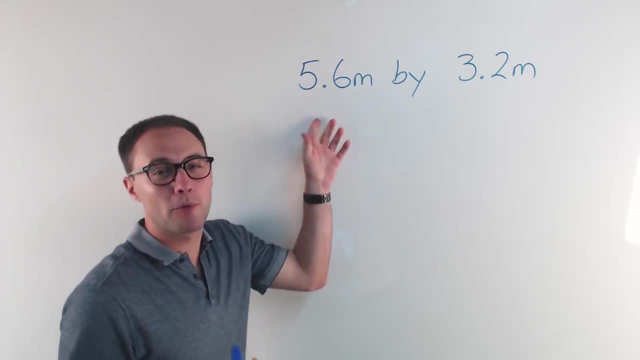 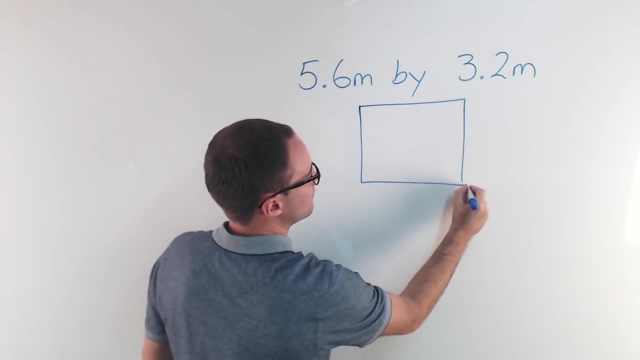 Alright, so let's talk about that wall. It was 5.6 meters by 3.2 meters, So if you think drawing a picture, you know this is going to be about 5.6 meters by 3.2 meters. 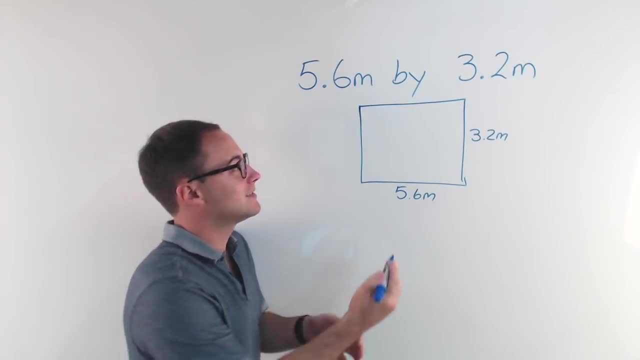 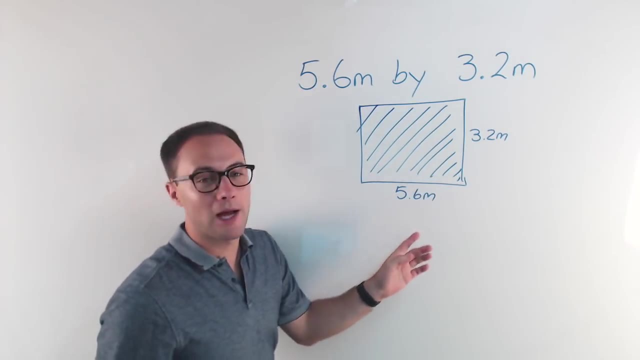 And we want to know if we're going to have enough paint. so what we need to find is the area, That's what we're covering with the paint. So to do that, we're just going to multiply right: Length times width. 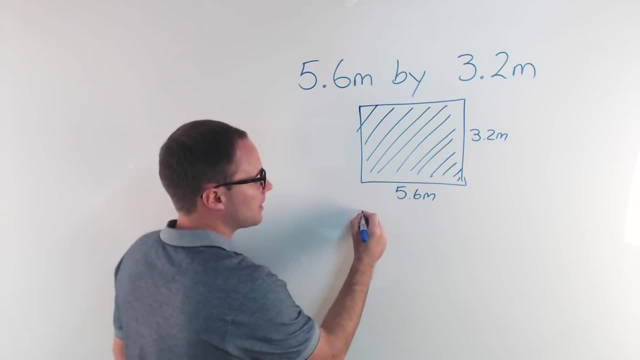 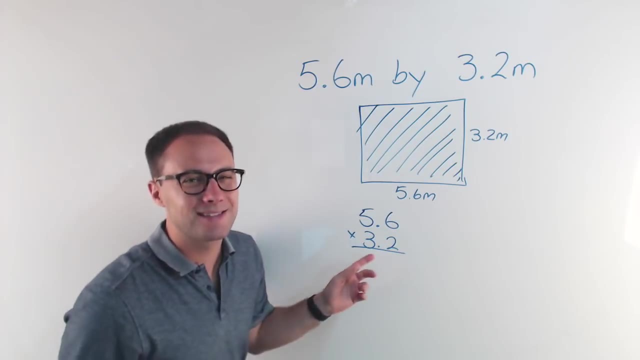 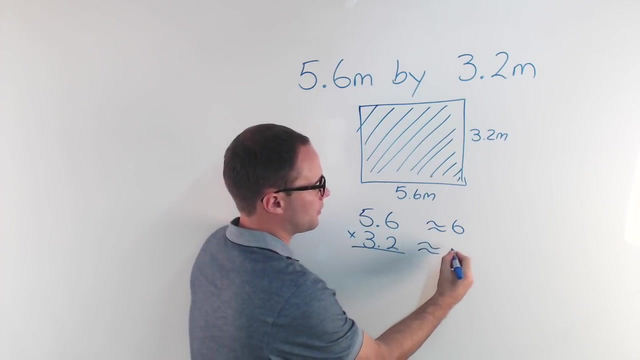 So 5.6 times 3.2.. 5.6 times 3.2.. Now, if we were going to estimate this, that would be about 6.. That would be about 3.. 6 times 3 is about 18.. So hopefully. 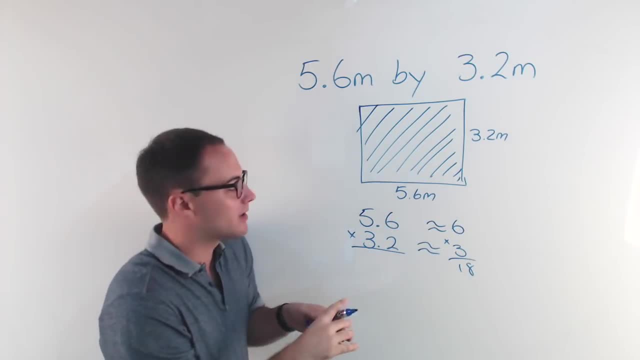 if our estimation is somewhere in accurate, we should have enough. So let's see, Let's just multiply 6 times 2 is 12,, 10, plus 1 is 11,. carry the 0, 18, another 1, 15 plus 1 is 16,, 2, 9,, 7,, 1.. 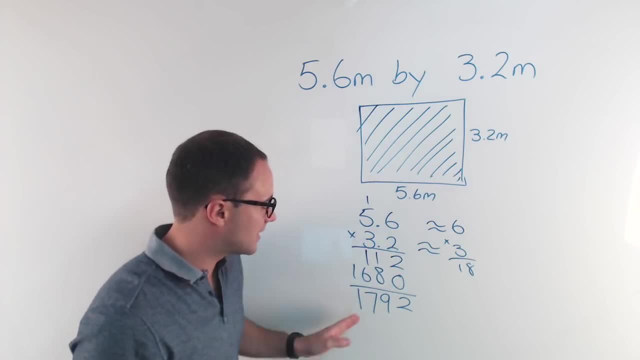 Now, if you're thinking well, where this is, decimals right. Where's my decimal point going to go? You think it should be close to 18?? Decimal point goes there: 17.92.. Don't forget your units. 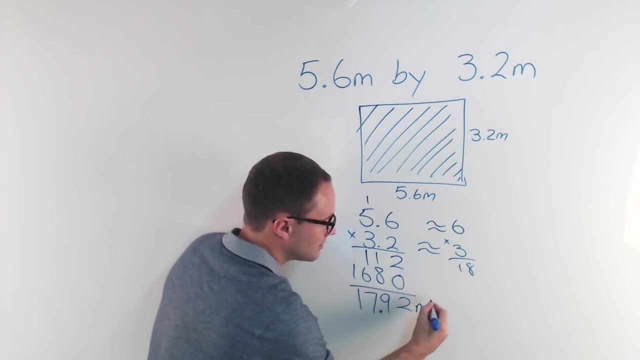 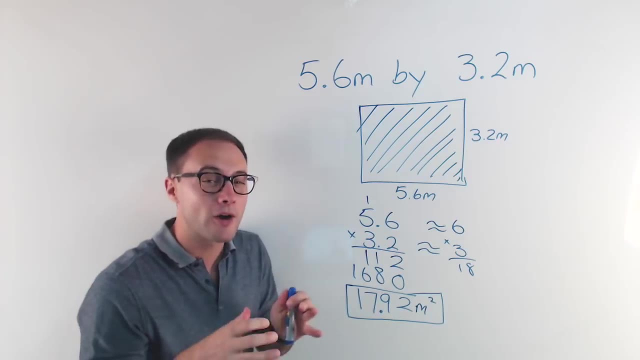 It was meters times meters, so that becomes meters squared, which makes sense for area, So 17.92 meters squared. The small can of paint could cover 20 meters squared or 20 square meters. So do we have enough? 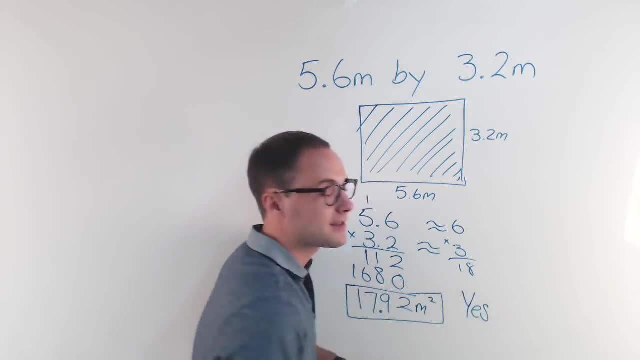 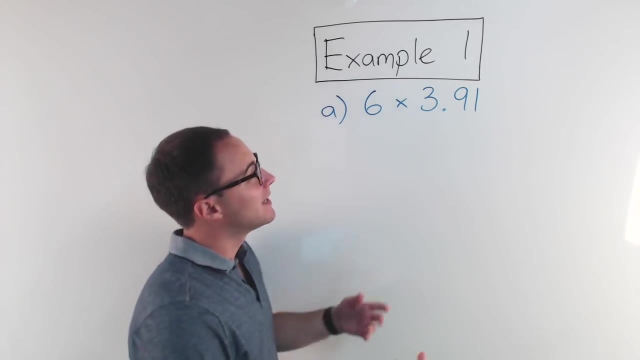 And the answer is Yes. Okay, So let's try another example. Alright, here's example 1. 6 times 3.91.. Now, when you're dealing with decimals, it's always a good idea to estimate. 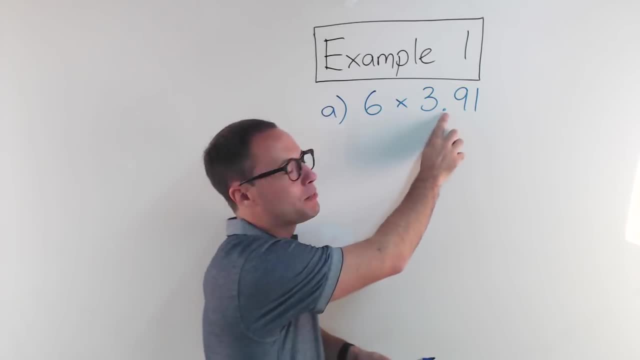 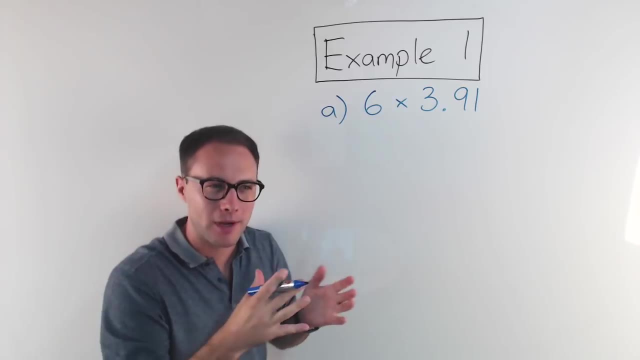 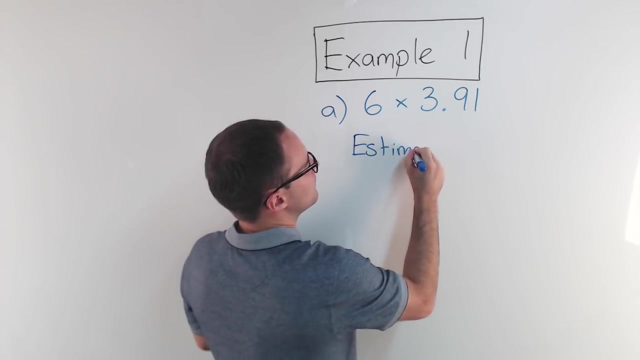 And the reason is because it can be very easy to put the decimal point in the wrong spot, which completely changes your answer. So if you estimate, that will help kind of catch those errors. So if we're going to estimate, this would be: 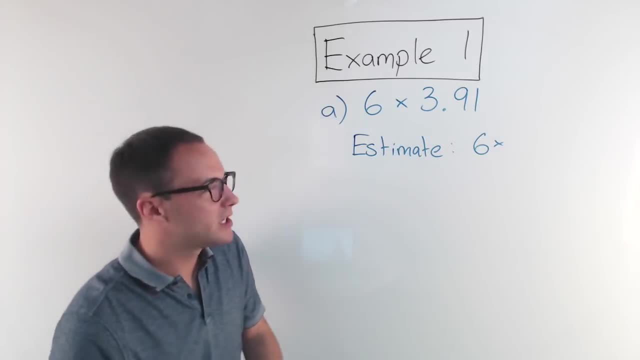 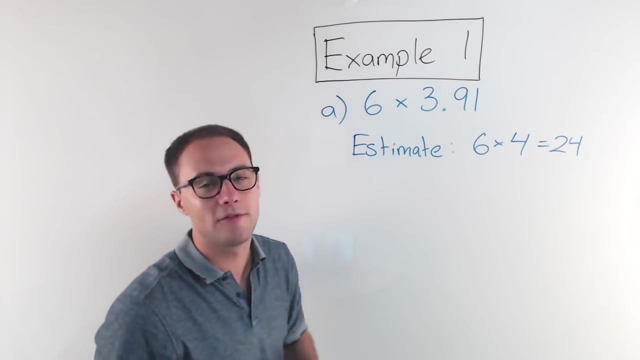 The 6 is okay: 3.91,. we can just round up to four, So we're thinking our product should be around 24.. So let's see Now, when you're multiplying with decimals, the trick is to treat it like the decimal isn't there. 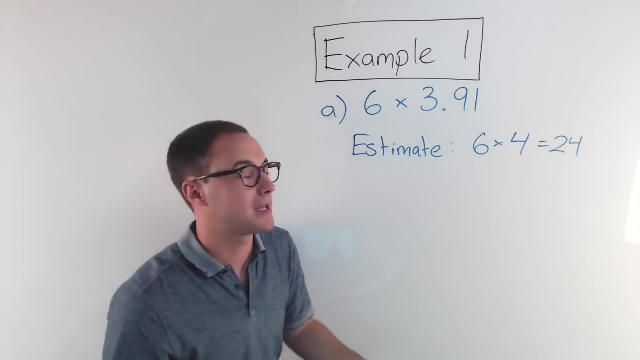 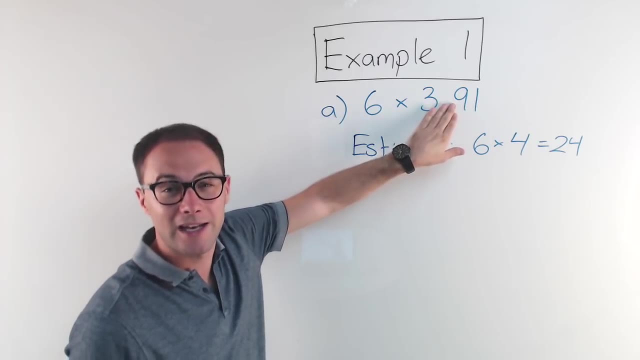 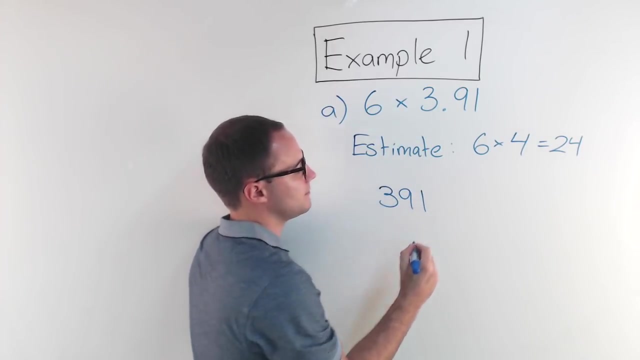 Set up the problem like you would, a normal multiplication problem. So what I'm saying is: don't think of this as 3.91.. Imagine it's just 391 times 6.. Well, if it was that, you would put the 391 on top, multiply it by 6.. 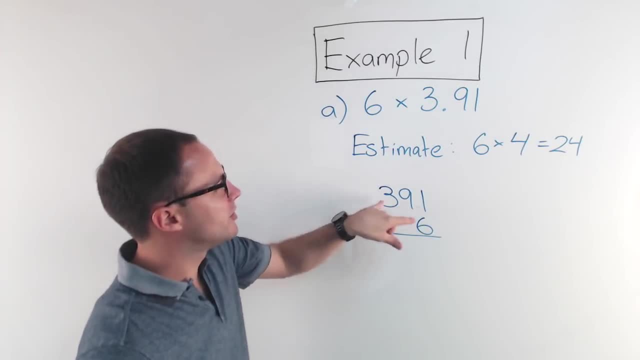 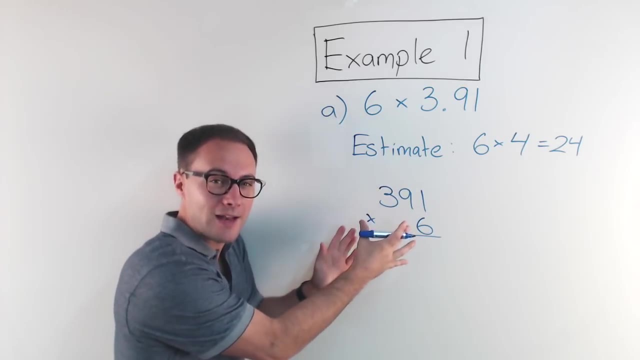 That's how you would set it up right, And we can do that, because order doesn't matter with multiplication because of the commutative property. So we can do that. Once you set it up like that, then go ahead and put the decimal point back in. 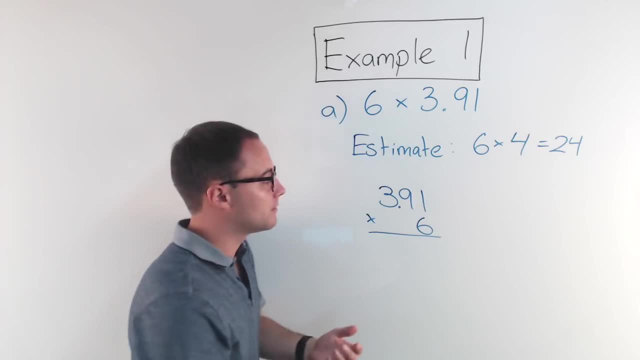 Just don't forget that. And now we just multiply like normal, That's going to be 6.. 6 times 9 is 54. Carry the 5. 6 times 3 is 18.. Plus 5 is 23.. 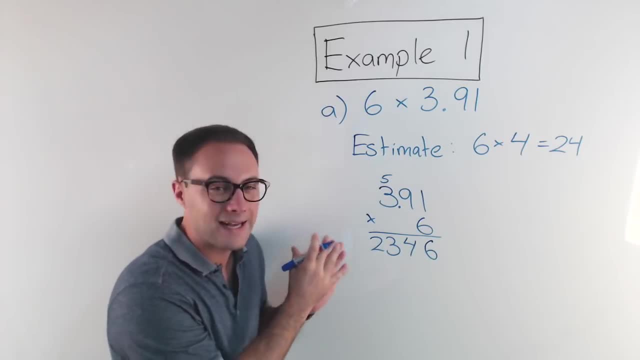 Now this is the last step And it's really important: Where does the decimal point go in our answer? And all you have to do is look at how many places you have after the decimal points in your problem. So here we've got the 9 and the 1.. 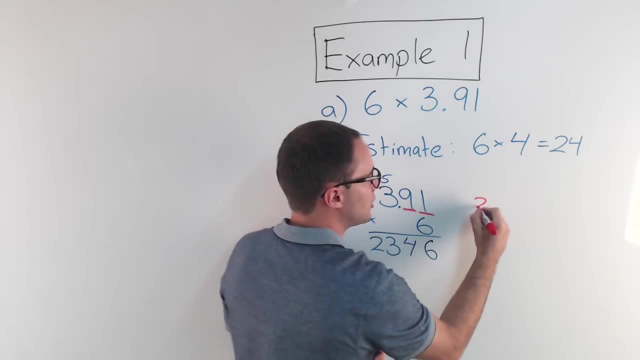 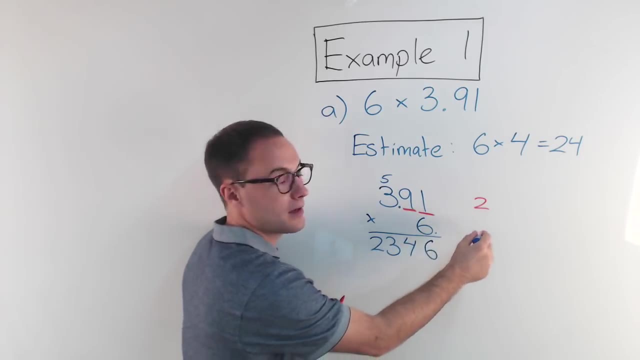 Two places after The decimal in 3.91.. So that's 2.. 6 doesn't have any right. The decimal point if we wanted would be here. There's nothing over there, So that's going to be 0.. 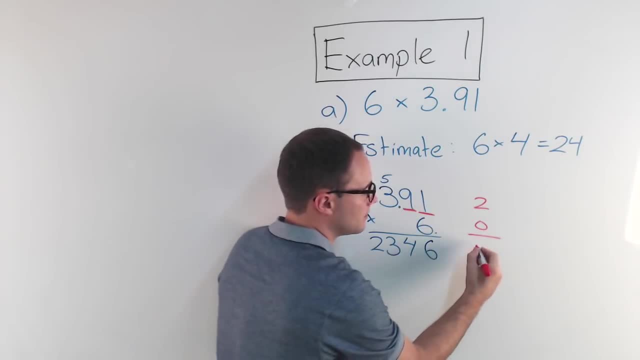 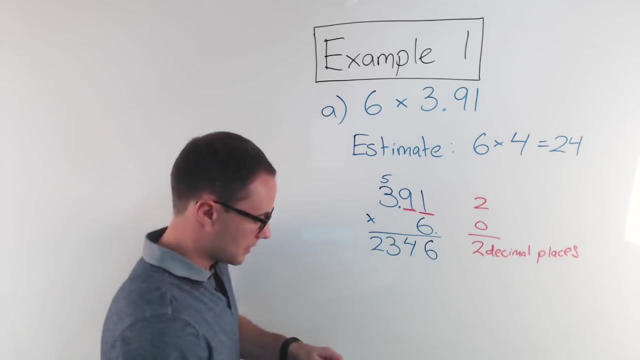 So in our answer we need two decimal places, So 1, 2.. The decimal point goes There And that is our product. That's our answer: 23.46.. And let's check: Does that make sense with our estimate? 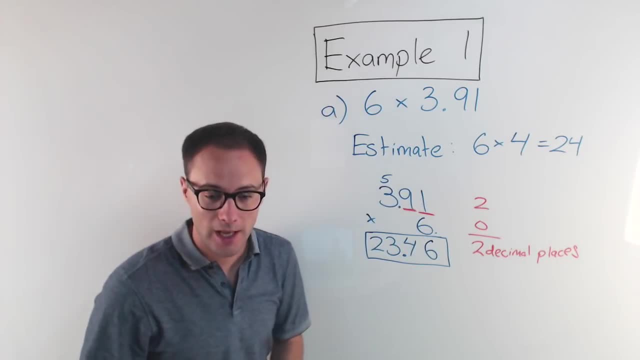 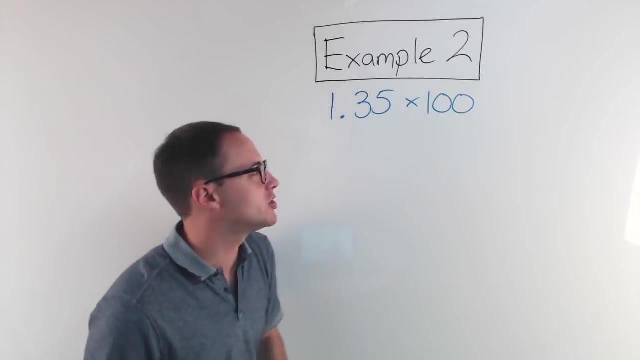 Yeah, it's really really close. So we know we're good. Okay, Let's try another one. Another example. All right, Here's example number 2.. 1.35 times 100.. When you're multiplying by powers of 10, like 100 is. 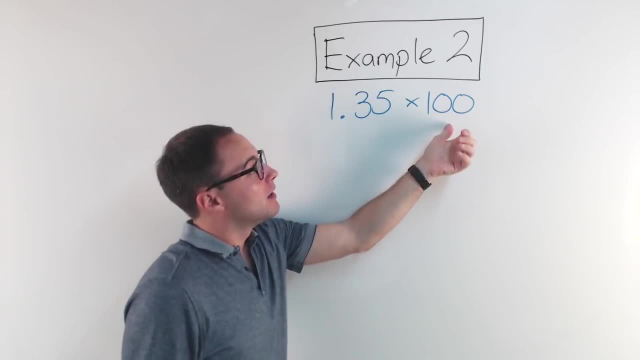 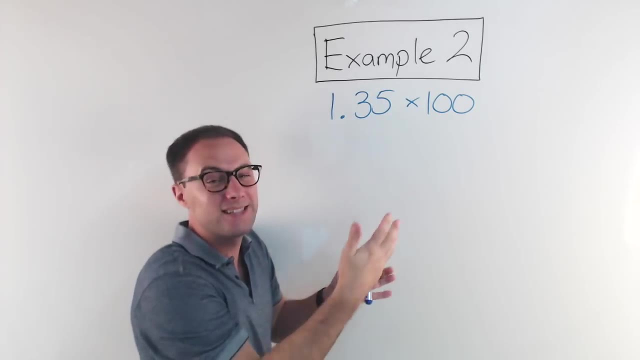 It's 10 times 10, right Or 10 squared. There's a really nice shortcut that you can make. If you remember, our whole number system is base 10.. It's based on powers of 10.. So if you think well, take it simpler. 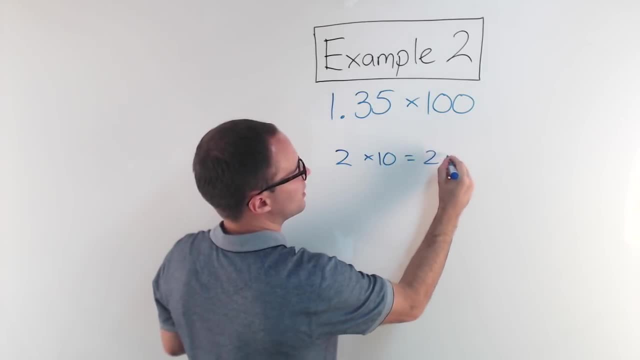 Well, what's 2 times 10?? Well, that's just 20.. 2 times 100.. That's 200.. 2 times 1,000.. Well, that's 2,000.. Okay, That's very simple. 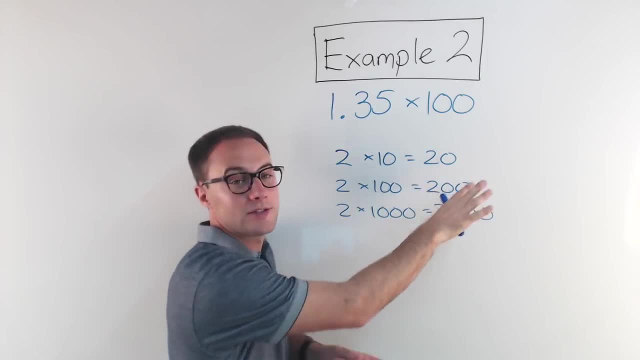 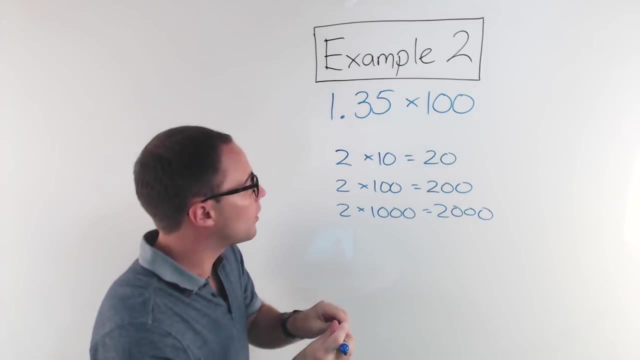 Okay, That's very simple, because it's just a whole number. All you do is add zeros at the end, right? You do the 1 times the 2 and then add however many zeros you have. But you can also think of it well, if there was a decimal here, where would it be? 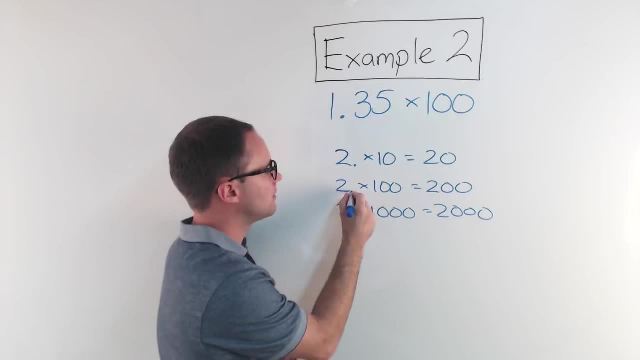 Well, with whole numbers, we can put a decimal right after. And now, from here to here. what happened to the decimal? It went from here over 1 and you just filled in a zero. Here it was times 100.. So we're moving it twice right? 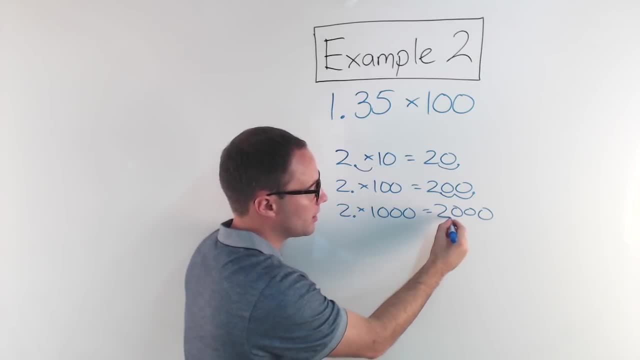 It filled in those zeros Here. times 1,000, you're moving the decimal point three times. When you're multiplying by powers of 10, you're moving the decimal point to the right And you just got to think: well, how many powers of 10?? 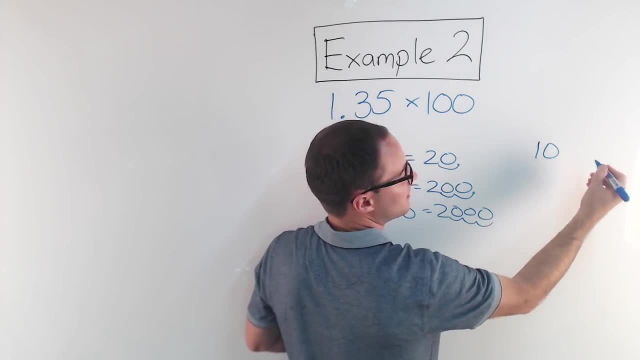 10, you're moving it once. 10 is the same as 10 to the first power. 100 is 10 squared, So you're moving it twice. 1,000 is 10 cubed: You're moving it three times. 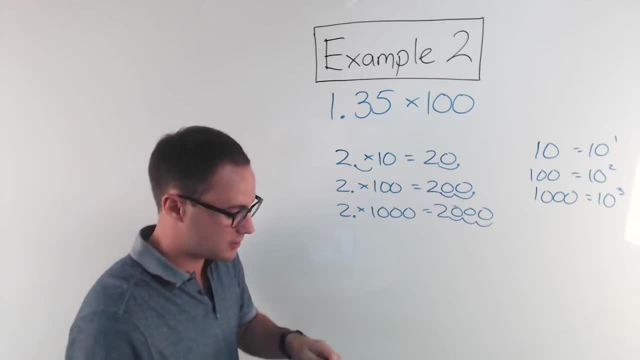 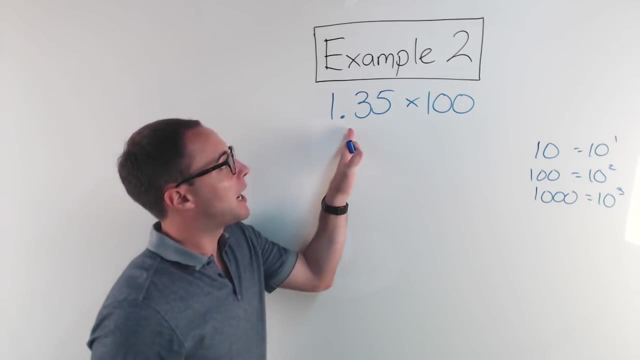 You can also think how many zeros are there, That's how many times you're moving it. So with that in mind, this problem becomes much, much easier. I'm multiplying by a power of 10.. I'm going to move it to the right because I'm multiplying. 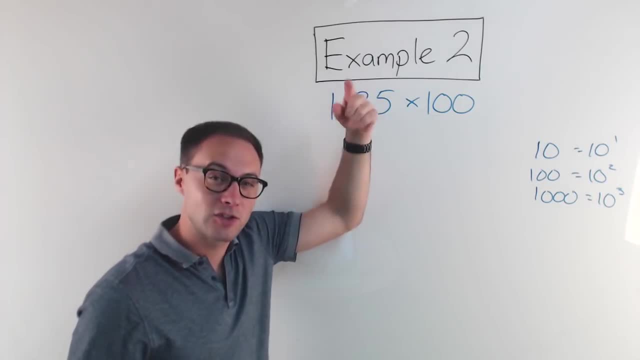 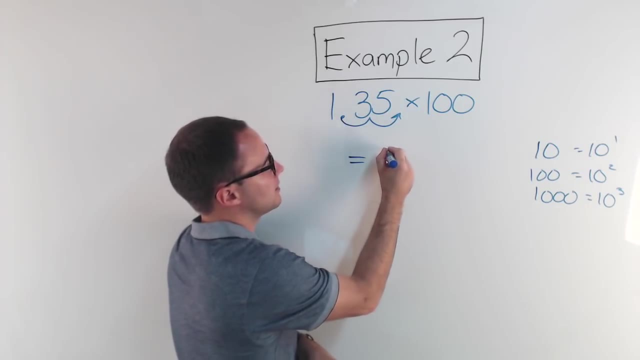 And there's two zeros, or I can think of that as 10 squared to the power of 2.. So I'm going to move it Once twice, So that becomes 135.. Very simple. Here's something to try on your own. 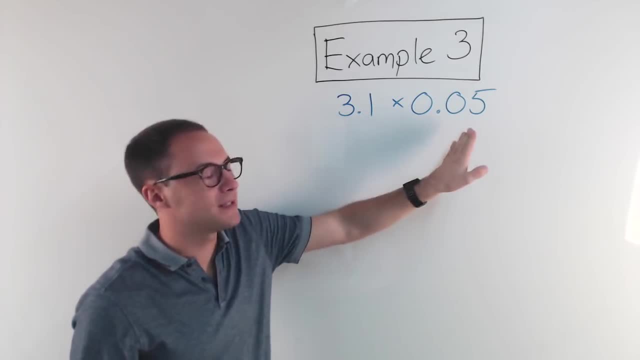 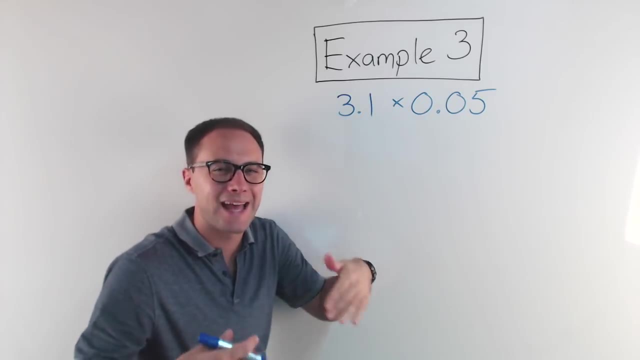 All right. here's our last example: 3.1 times 0.05.. Now, if you remember, at the beginning of the video I said, when you're multiplying with decimals, pretend the decimal points aren't there and set up the problem like that. 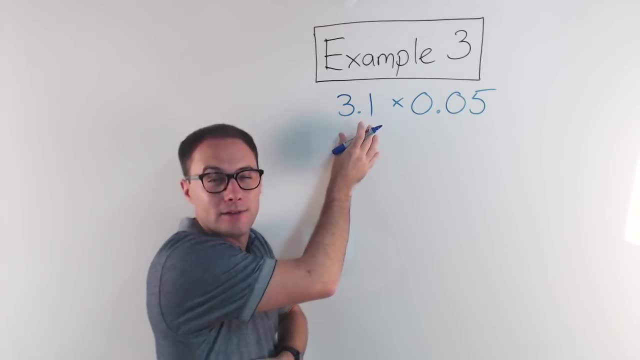 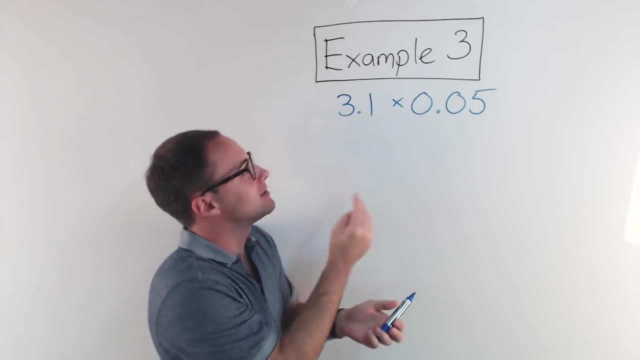 So I'm not going to think of this as 3.1. I'm going to think of it as 31 times 0.05.. Now there's a couple of ways. I could put the 31 on top, or I could put the 0.05 on top. 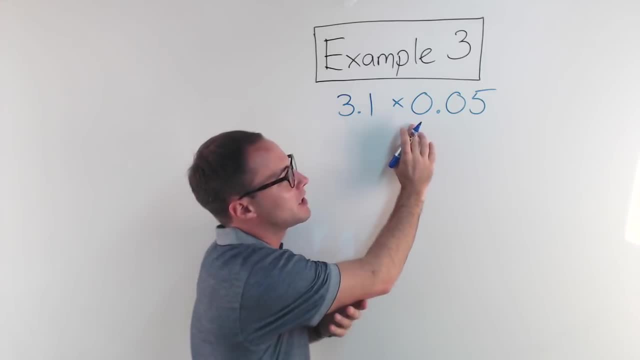 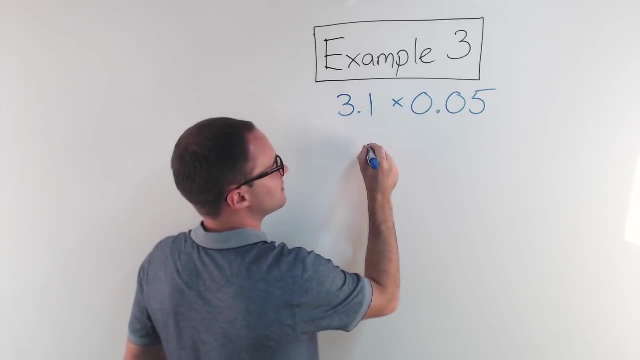 Me personally. I like to do whichever ones have the most digits. I like to put that on top, But it doesn't matter, You can do it either way you want. So I'm going to set this up as 0.05 times. 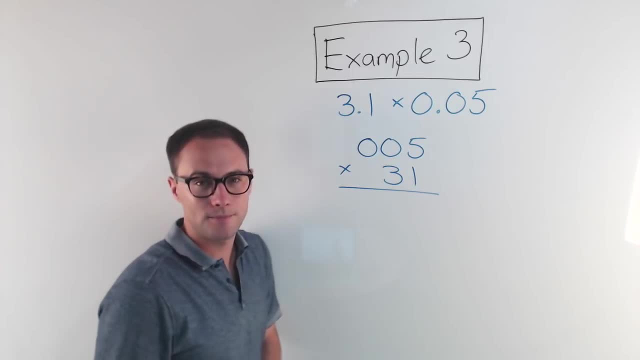 31. Pretend the decimal points aren't there and set it up that way. Now that I've set it up, I'm going to put them back, so I don't forget. Decimal point is there. Decimal point is there. Now you'll notice these decimal points aren't lined up. 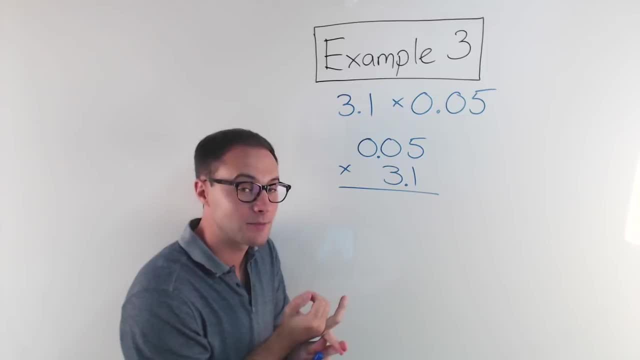 And that is the main difference between adding and subtracting decimals, where the decimal points have to be lined up, and multiplying with decimals where they don't. That's the main thing to remember, So you should write that down. When you're multiplying with decimals, the decimal points do not have to be lined up. 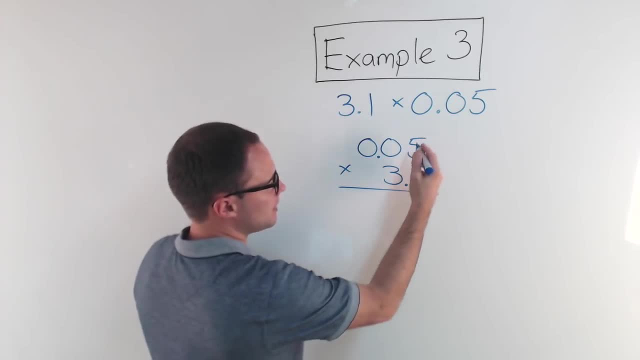 So that's how we're setting it up, And now I just multiply: One times five is five. That's going to be zero, zero. Add a zero Three times five is 15.. Carry the one That's zero Plus one is one.